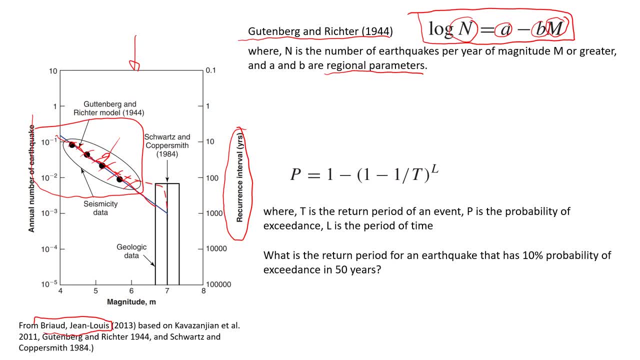 It's a log scale, The original data devised by Gottenberg and Richter- that only use annual number of earthquakes. that comes here from this formula. You see that so that if you want to actually estimate how long it's going to take to stronger earthquake to occur, we're going to use what is called characteristic model. 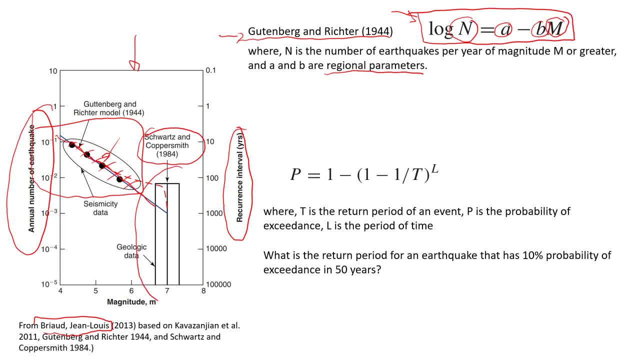 developed by this researcher. So this part of the chart. So you see that for this particular, for earthquakes which are greater than six, we also need to consider geologic data such as false length and historic sleep rate. So in this particular case, that's what we need to do. 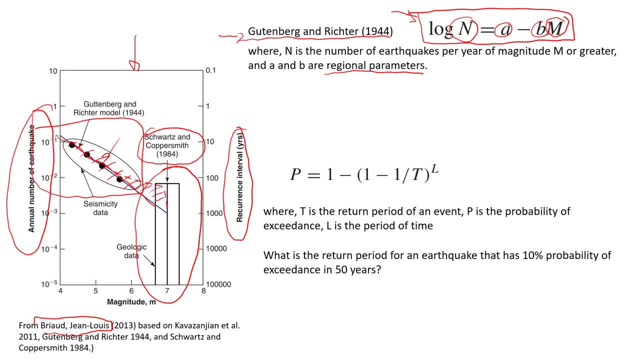 and this will be a little bit improvement compared to the Gottenberg-Richter model. So now let's see how we can use it. For example, if we have a magnitude of six, how long it's going to take to occur for this particular earthquake? So we're just going to look. 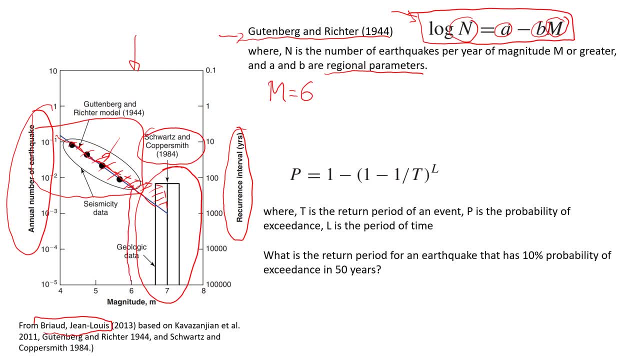 at and we're going to look that magnitude six is here, So we can still use this exponential line of the Gottenberg-Richter model, and then it's going to give us number here, So this will be log scale. Unfortunately, in this chart you don't have this little marks. 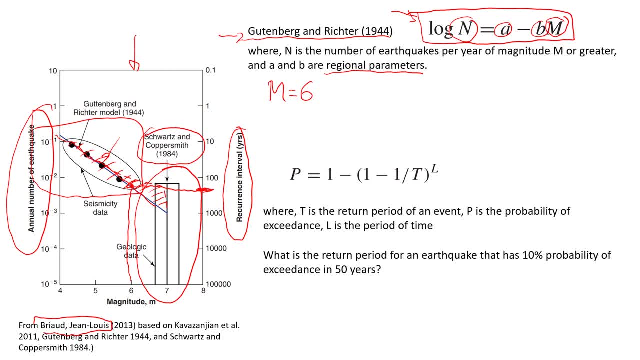 for log scale, So we have to have some estimation. So because this is log scale, we assume that it's about 200 years. So we can estimate that for approximately 200 years. So please remember that it's not going to give you exact number, exact estimate. It just give you. 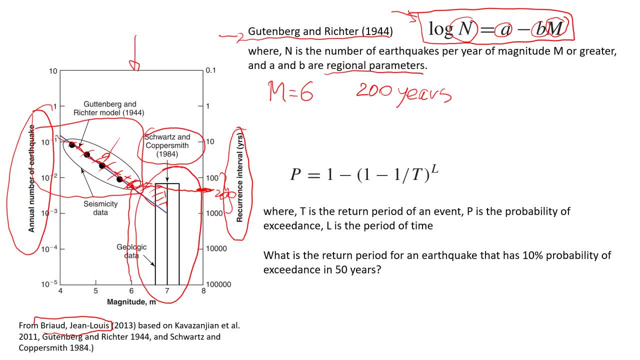 some approximation how long it may take for this particular earthquake to take place. right, And if you look at again at this chart, you will see that if there's a relatively weaker earthquake with relatively smaller magnitudes, they're going to happen more often. 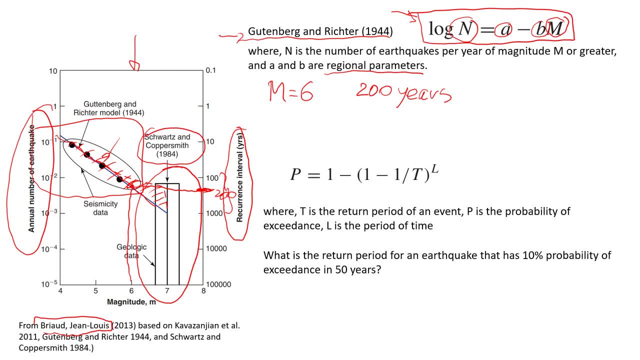 compared to the earthquakes with very high magnitude, For example, for the earthquake that just took place recently in Turkey, in Syria, so that the value was, the magnitude was more than seven. So this actually doesn't even provide good estimates because it's very difficult. 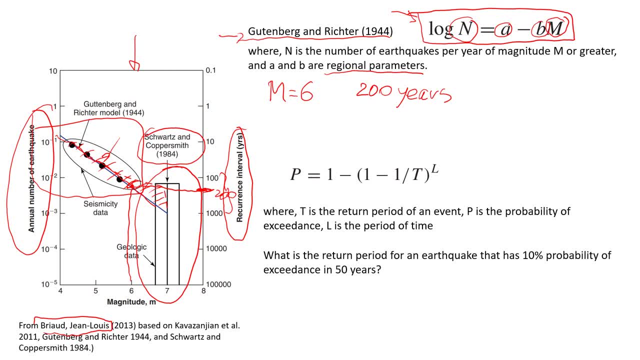 to estimate how long it's going to take, But let's say even was about seven. So somewhere in this area, I believe from 500 to 1000 years to take place. Okay, so this is just to give you some idea how you can get some quick estimation of earthquake reoccurrence. And now let's look at probabilities. 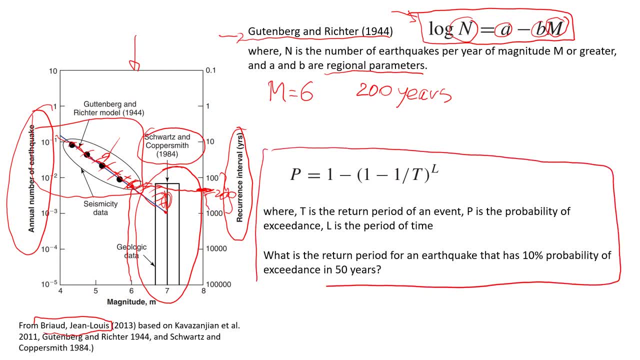 So how we can use probabilities and how we can also estimate the return period of this particular event or earthquake. So you see that P in this formula is probability and T is the return periods- And usually we use it in years- and sorry, not years- and L is the period of time, So L is going to be years. 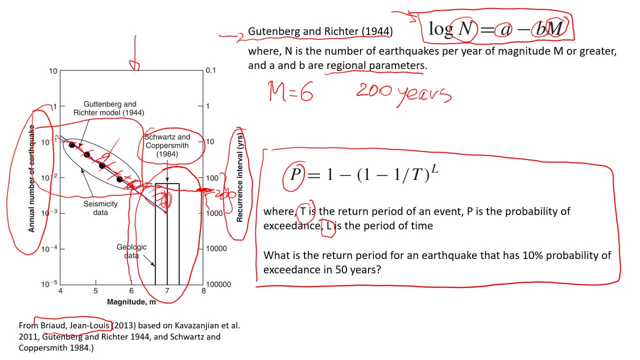 So now let's see how we can use this formula to estimate the return period of an earthquake that has 10% probability of exceeding some 50 years. So it's one in 50 years. So we can see that there is one in 50 chances that this particular day that there would be. 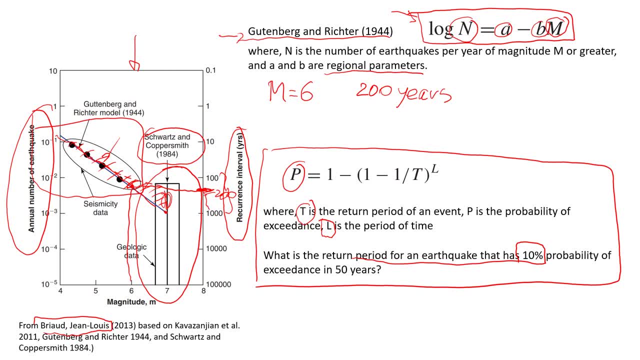 earthquake that would exceed this magnitude in the next 50 years. So what we're going to do, we will rearrange this formula for T, because that's what we need to get. So if we arrange the formula, we're going to have something like this: equal one divided by. 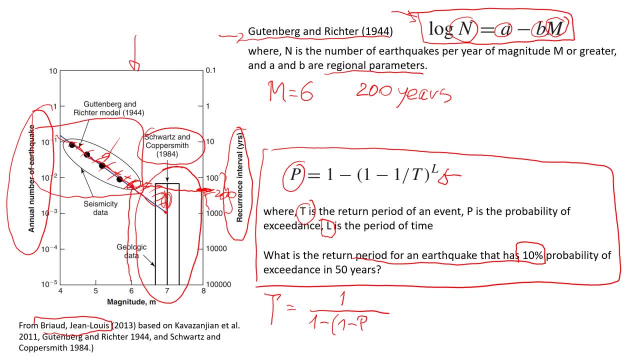 one minus one minus P power, one divided by L. So now if we put numbers here, we're going to have that we have 10% of probability. So here we still have one. Here we have one minus one minus P, So we would have 10% probability. However, the probability is 10%.